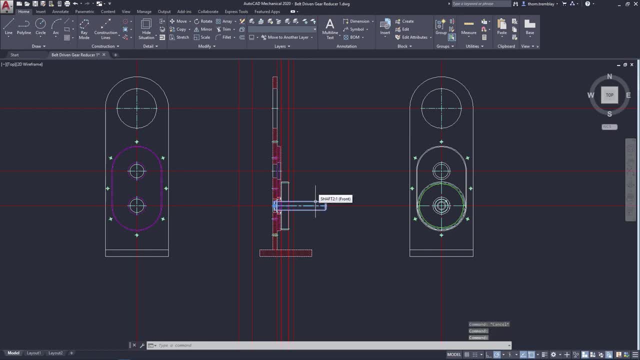 versions of AutoCAD emerged for architects, electrical controls engineers and mechanical designers. While these tools were powerful and added additional performance, they were also a great way to improve the performance of the design, In addition to the additional productivity. not everyone took advantage of them, or was. 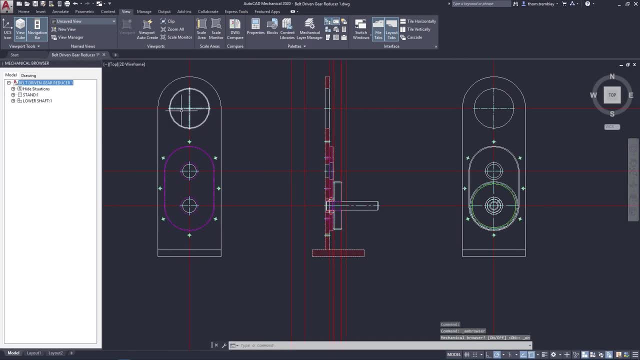 able to transition to these tools With one AutoCAD. all of these tools are available to anyone using the current release of AutoCAD. In this collection of videos, we will see a handful of the tools that make AutoCAD Mechanical such an incredibly productive tool. Some of 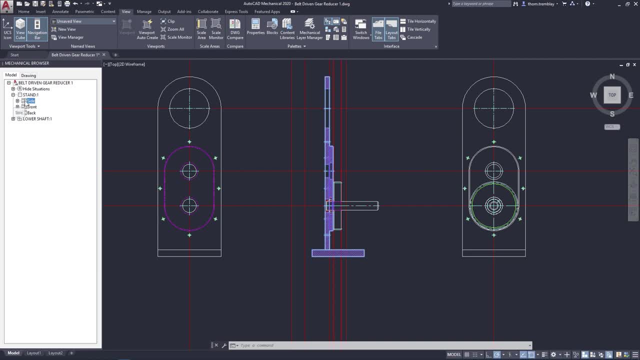 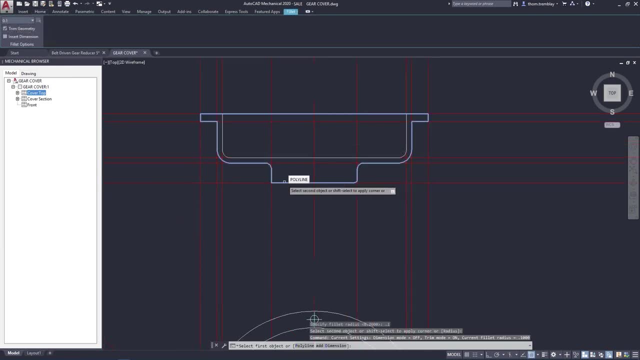 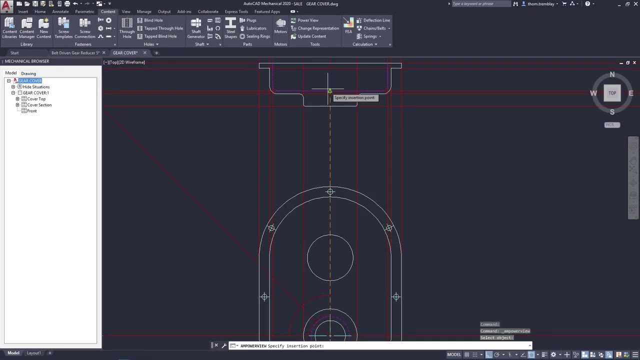 these items will include looking at how AutoCAD Mechanical can organize data in a 2D drawing based on the component structure of a design. How AutoCAD Mechanical is able to take tools that are already in regular AutoCAD and add additional functionality, such as using construction lines to create projected views. 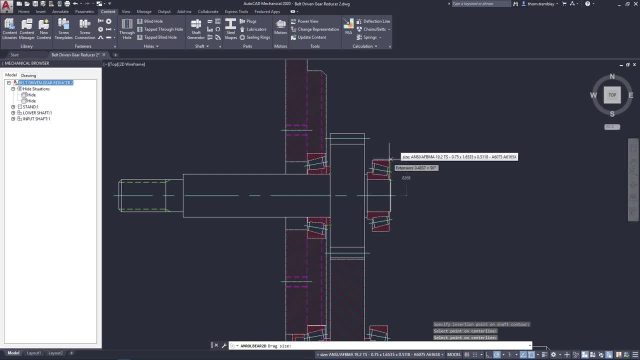 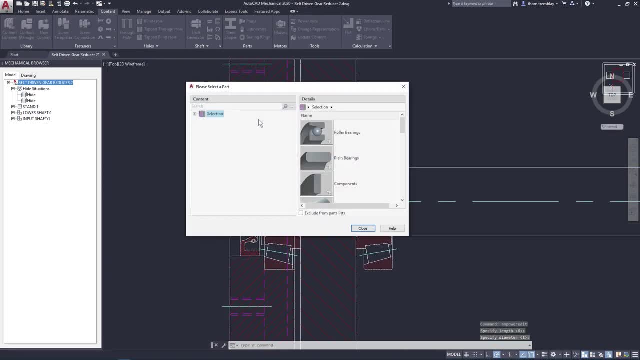 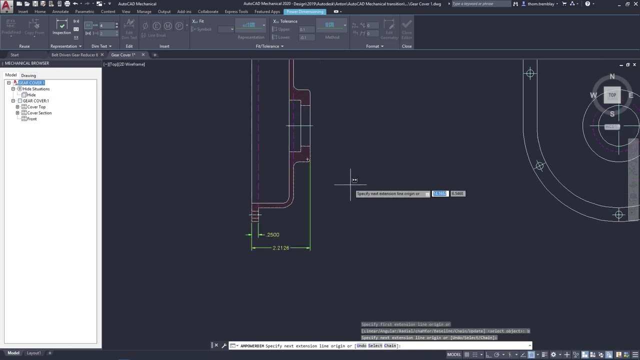 Standard components are everywhere inside of AutoCAD Mechanical, with access to bolts, bearings and other machine components, just scratching the surface of how they can be used. In AutoCAD Mechanical, you can also move beyond the creation of the basic geometry to fantastic detailing tools, Everything from smart power dimensions to mechanical-specific 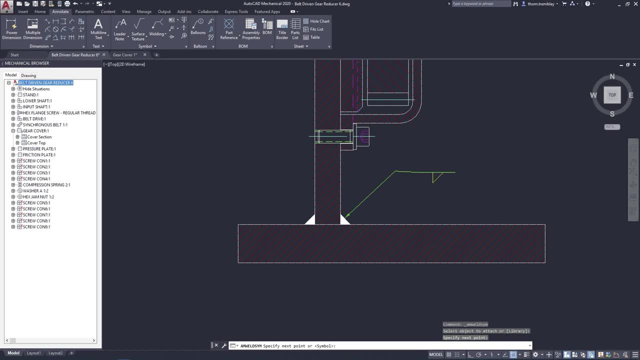 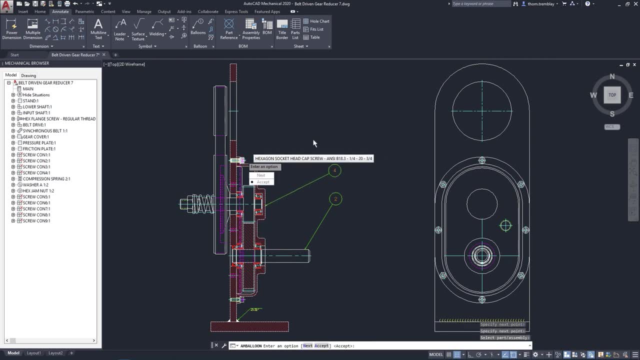 detailing and callout tools. All of this together will ultimately lead to your ability to apply intelligent balloons and generate parts lists that stay in sync. As you watch these videos, I'll ask you to reflect on how much time you're spending and how many steps you're taking to replicate the outcome that AutoCAD Mechanical is able. 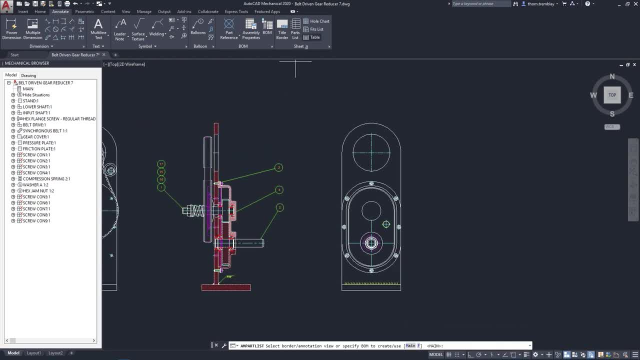 to deliver in just a few seconds with AutoCAD Mechanical. Thank you for watching this video. I hope you enjoyed it. If you have any questions, please feel free to ask them in the comments below. After seeing how incredibly productive AutoCAD Mechanical is, install it for yourself and. 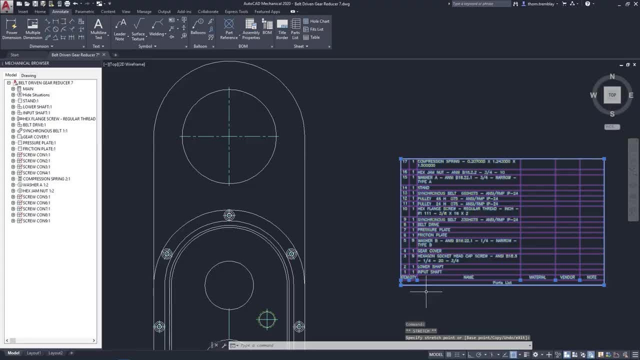 begin the process of learning just how powerful AutoCAD can be.